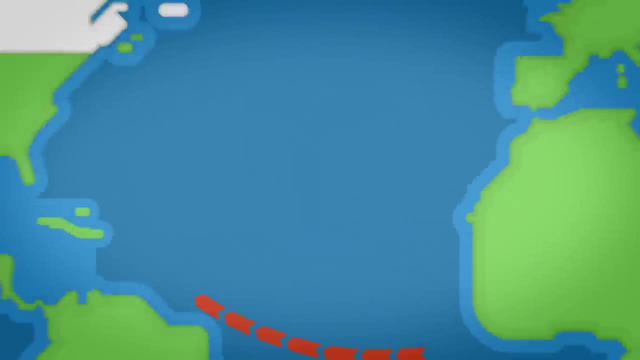 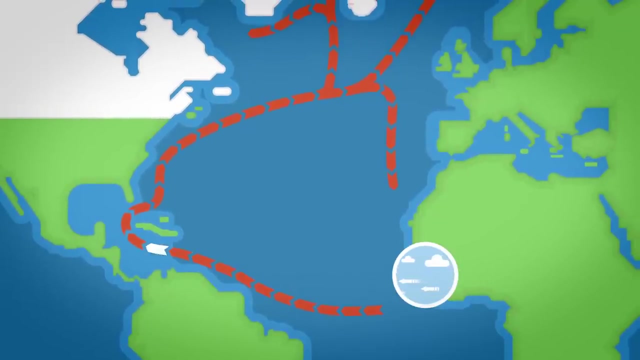 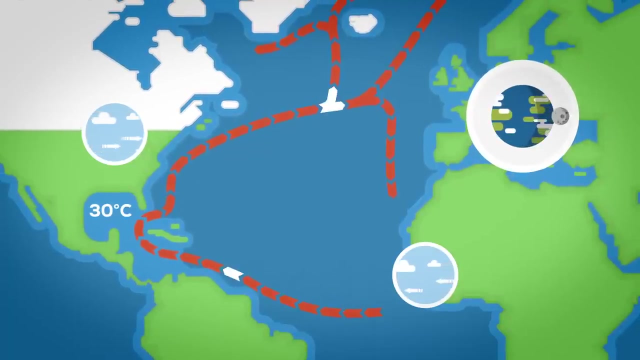 A constantly blowing wind. the Southeast Trade Wind drives warm water to Europe. This wind drives warm surface water to the northwest, into the Gulf of Mexico, where it heats up to 30 degrees Celsius. The turning of the Earth and the west winds then direct the Gulf Stream towards Europe and split it up. 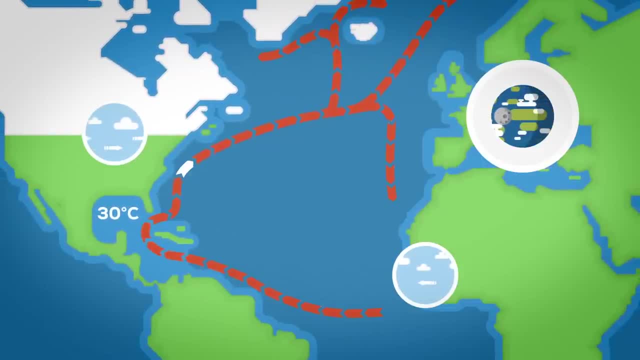 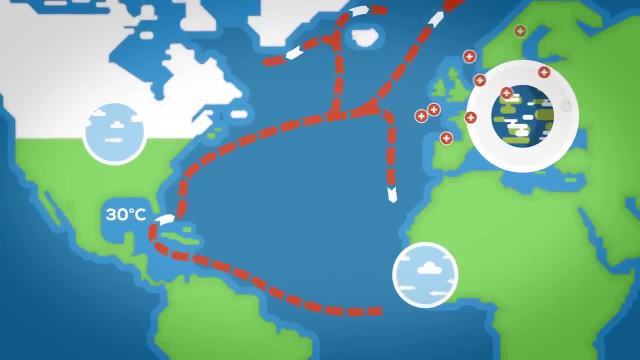 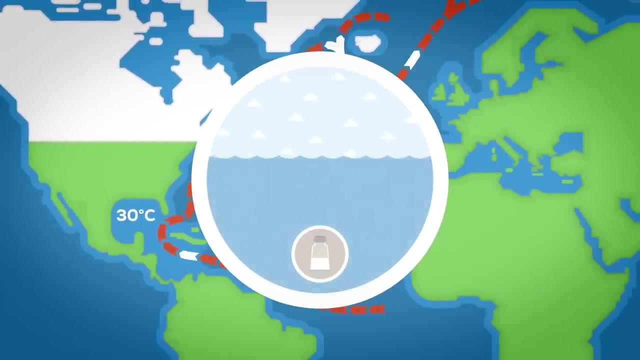 One part flows south, another east, to the Canary Current, and a third part flows north, where it releases a lot of heat into the atmosphere. as the North Atlantic Current. The water becomes colder there, Its salt content and density rise on account of evaporation, and it drops down between Greenland, Norway and Iceland. 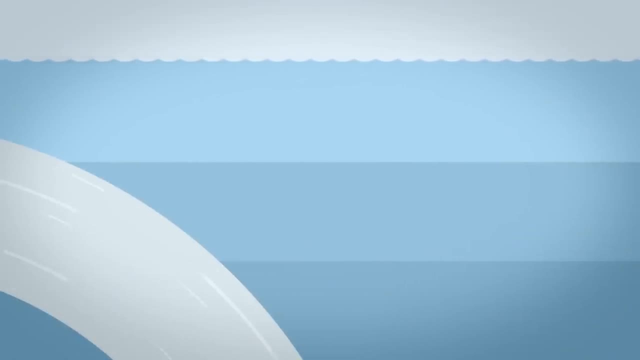 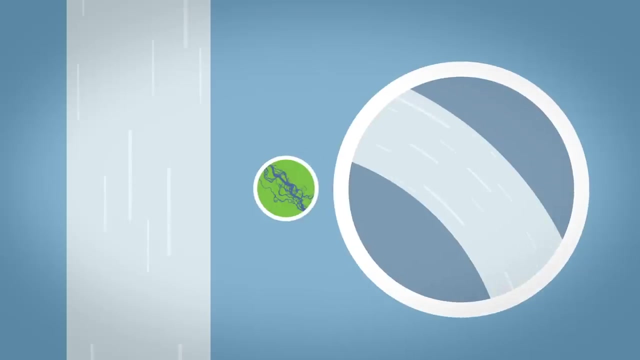 There we also find the largest waterfall on Earth, the so-called chimneys- Roughly 15 kilometer wide pillars with water falling up to 4,000 meters. 17 million cubic meters of water per second, or roughly 15 times more water than is carried by all the rivers in the world. 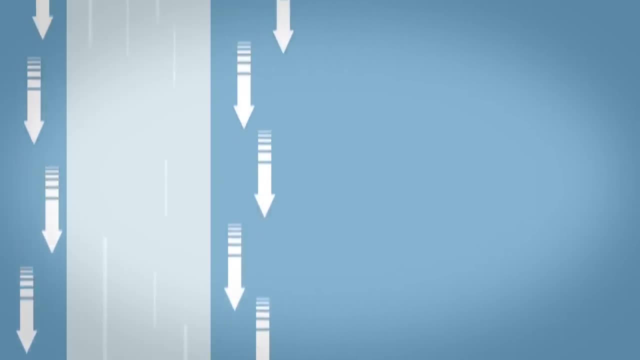 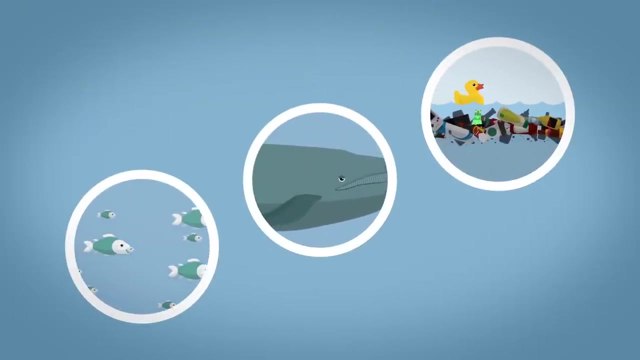 This creates a strong maelstrom Which constantly pulls in new water, and is the reason that the Gulf Stream moves towards Europe. Countless species use the Gulf Stream as a means of transport on their trips from the Caribbean to northern areas, But it doesn't just bring us animals. 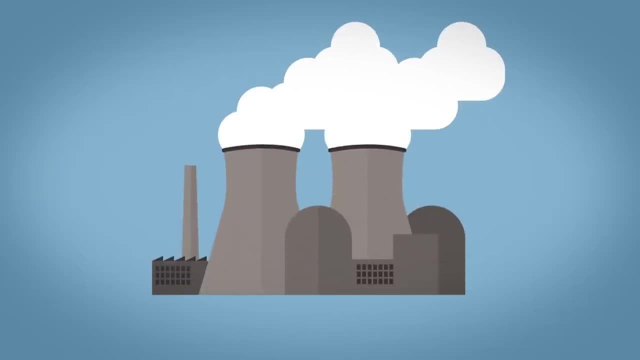 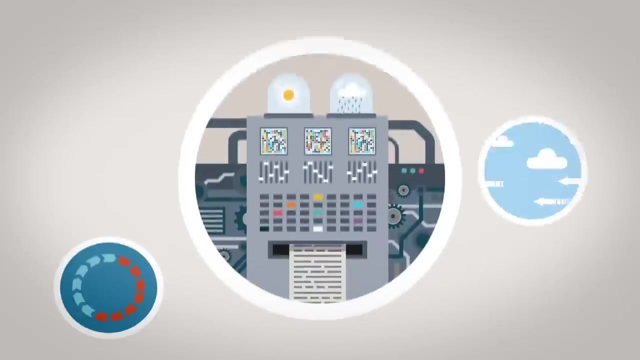 An enormous quantity of warm air also comes with it. In order to reduce the same heat which it brings to the shores of Europe, we would need one million nuclear power plants. That's why we also call the Gulf Stream a heat pump. Without it, the temperature would be significantly colder here. 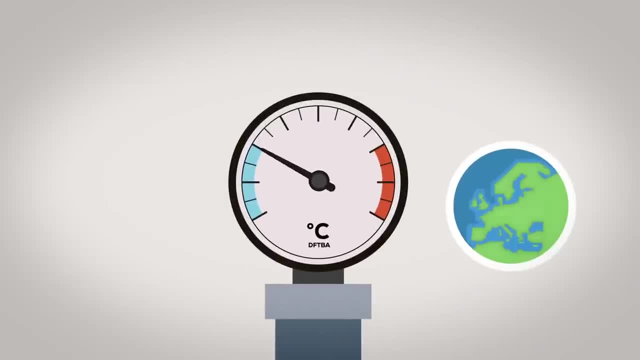 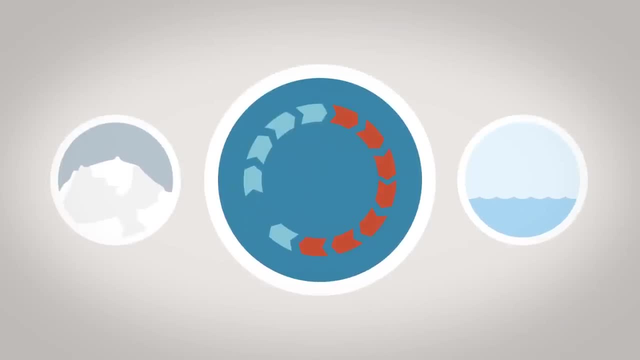 At least 5 to 10 degrees. Instead of lush fields, we would have long winters and sparse, ice-covered landscapes in Europe. In the last few years, scientists and pundits in the media have repeatedly expressed the fear that the Gulf Stream could come to a standstill due to climate change. 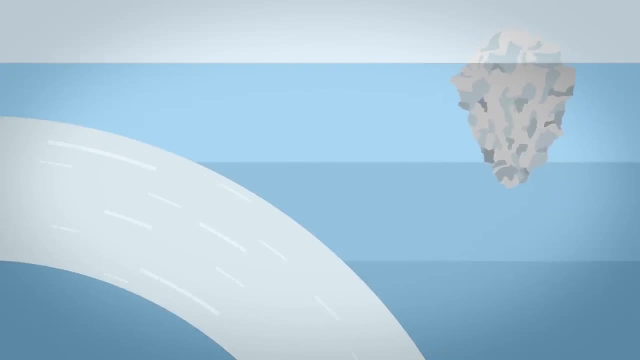 Because if the polar caps actually melt, the salt content in the water off Greenland would fall, as would its density. The North Atlantic current would no longer be heavy enough, and so it wouldn't sink as usual. In the worst case, that would bring the Gulf Stream, our heat pump, to a stop.